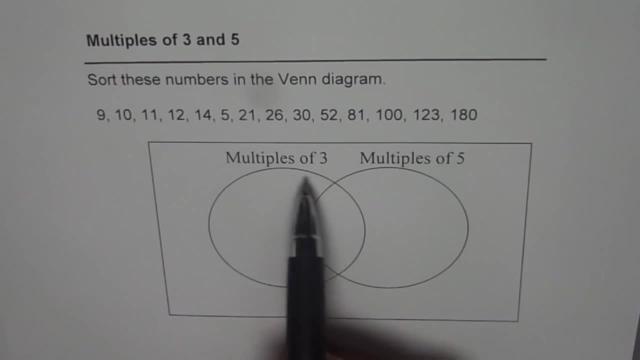 Now in this Venn diagram. here you have to put multiples of 3 and the second one is for multiples of 5.. You can pause the video, solve the question. then look into my suggestion And what goes inside. These are the numbers which are multiples of both 3 and 5.. The common multiples of 3 and 5 will go here, Right? So let's begin One by one and then place these numbers in the Venn diagram. 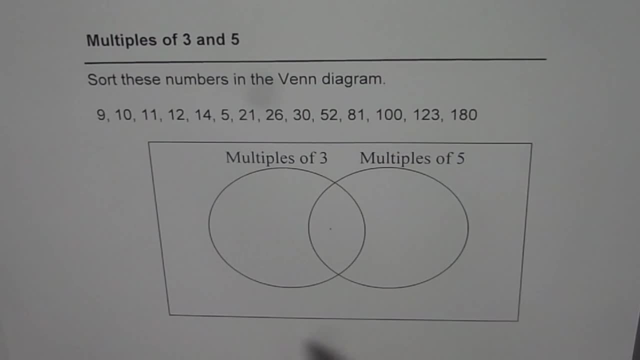 So now 9.. 9 is a multiple of 3.. Is it a multiple of 5?? No, it is not. How do you know? Well, multiples of 5 should end with which numbers? Should end with 0 or with 5.. Correct, So that is multiples of 5.. Is it ok? 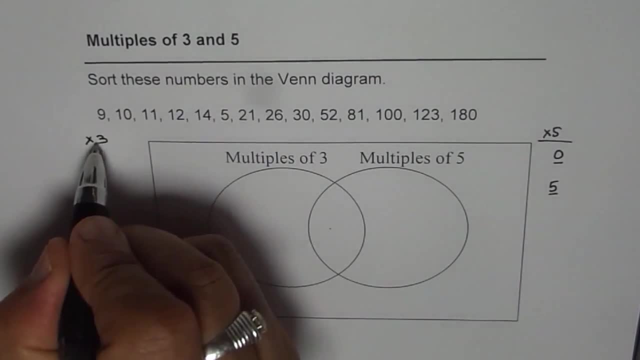 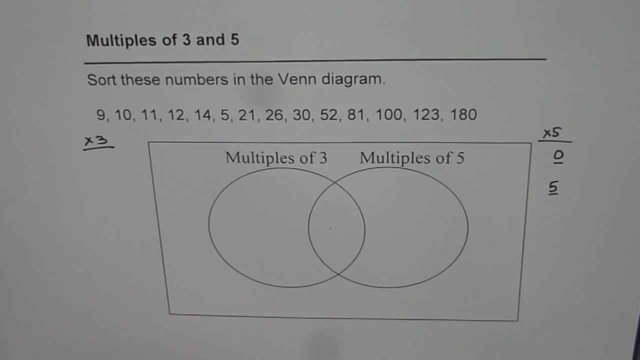 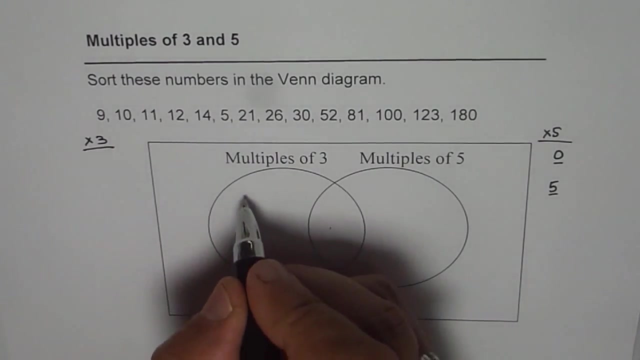 How about multiples of 3?? What is the rule For 3,? when you add the numbers that should be divisible by 3.. That's a simple rule. Ok, So we'll use this rule and then place the numbers 9.. 3 times 3 is 9, and 9 doesn't end with 0 and 5.. So 9 is just a multiple of 3.. It comes here, So we'll write 9 here, Correct? 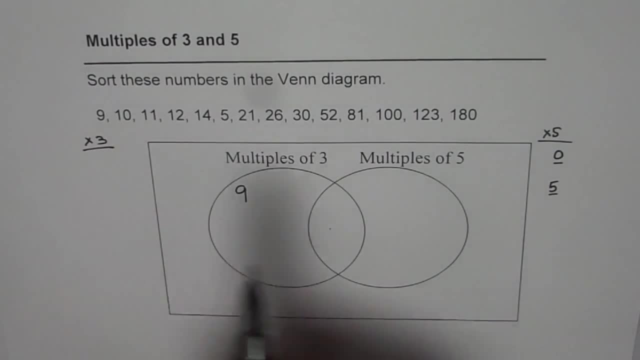 10.. 10 is not a multiple of 3, but it is a multiple of 5.. It ends with 0 or 5.. So 10 comes. on the other side, 11 is prime number. It is not a multiple of 3 or 5. So it comes outside. So we'll write here: 11 outside. Do you understand? That is how you have to place your numbers. 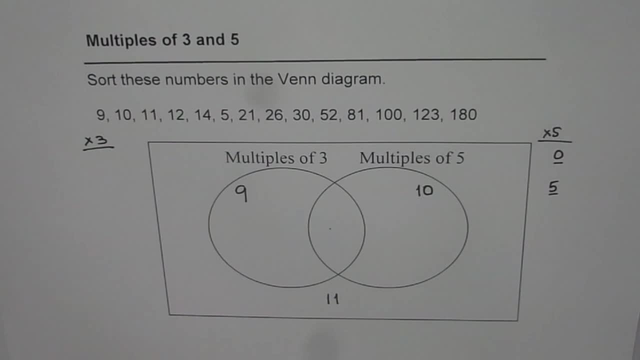 Now you can pause the video and place all the numbers at the right place and then check with my answer. That would be a good exercise to do. Let's continue. 12 is 1 plus 2 is 3.. It comes here Right. Let me write 12 here. 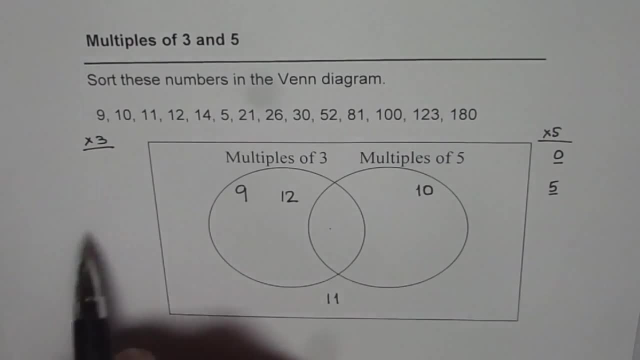 14.. 1 plus 4 is 5.. It cannot be divided by 3.. Now does it end with 0 or 5?? So 14 comes outside. 5 is a prime number, but it is a multiple of 5.. So I should put here right, Not there. I was about to make a mistake.